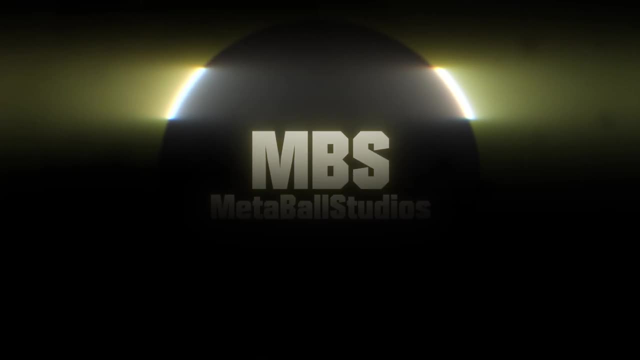 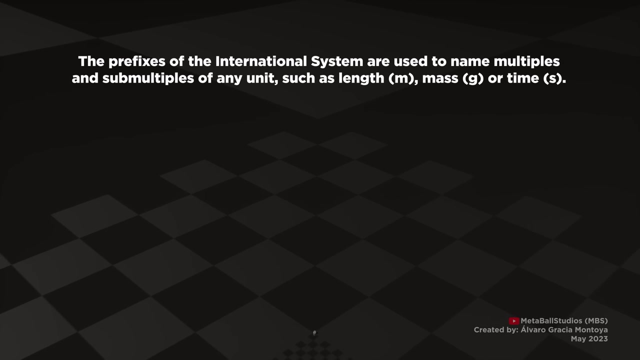 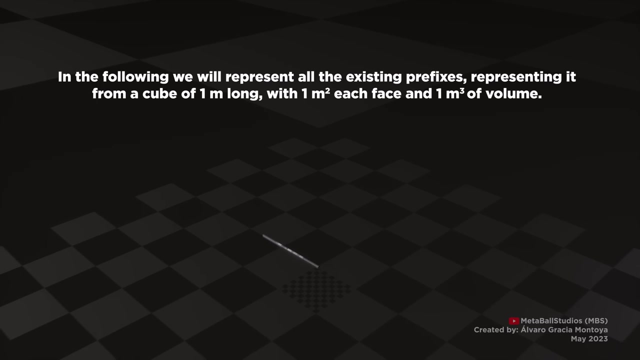 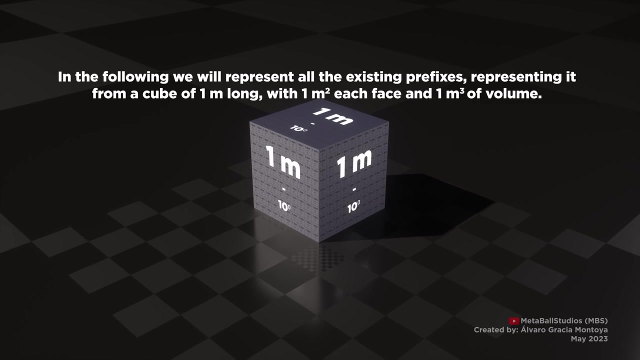 The prefixes of the international system are used to name multiples and submultiples of any unit, such as length, mass or time. In the following we will represent all the existing prefixes, representing it from a cube of one meter long, with one square meter each face and one cubic meter of volume. 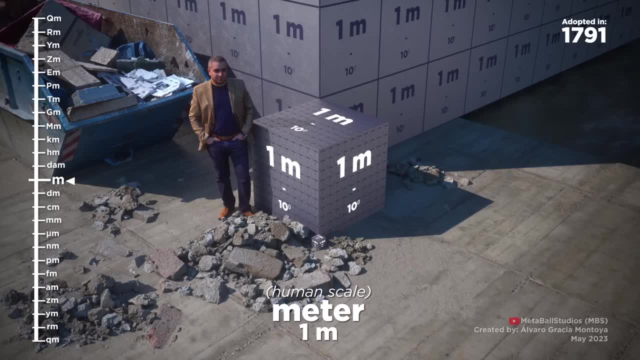 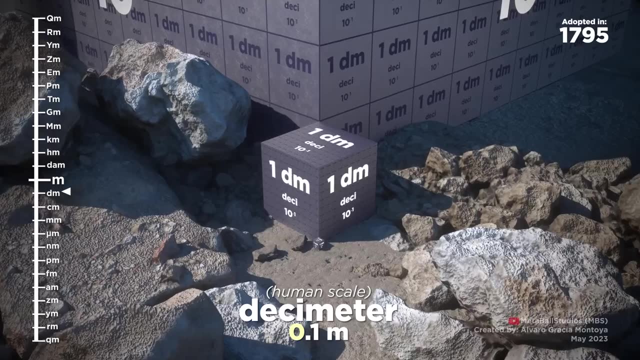 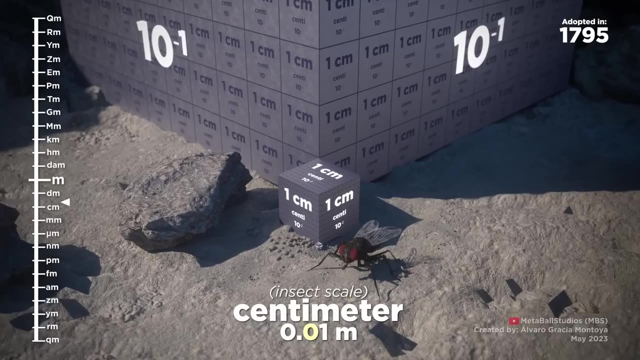 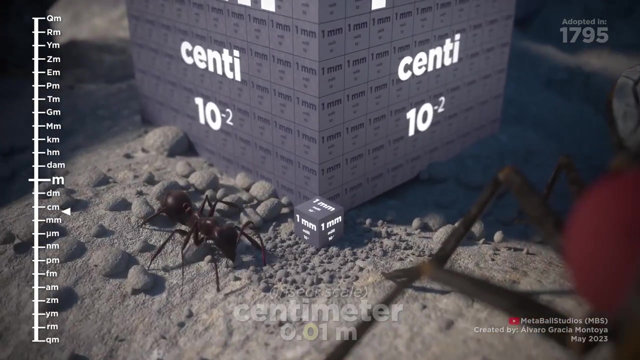 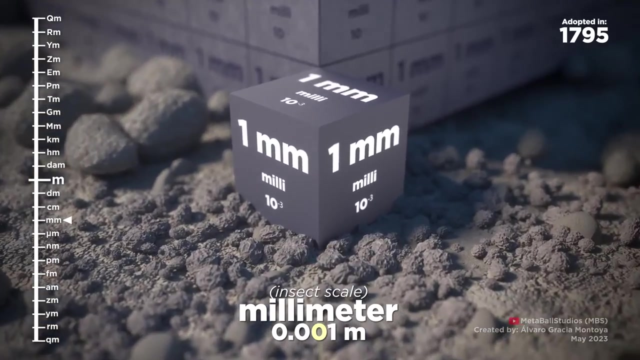 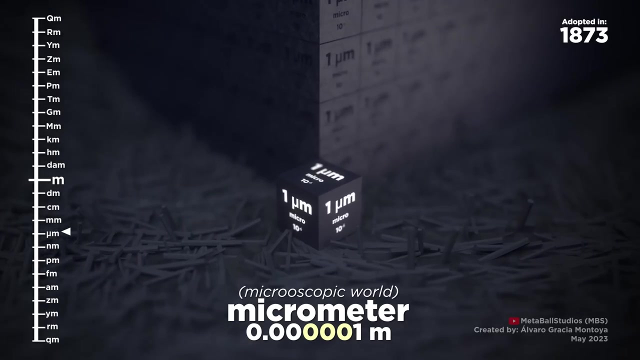 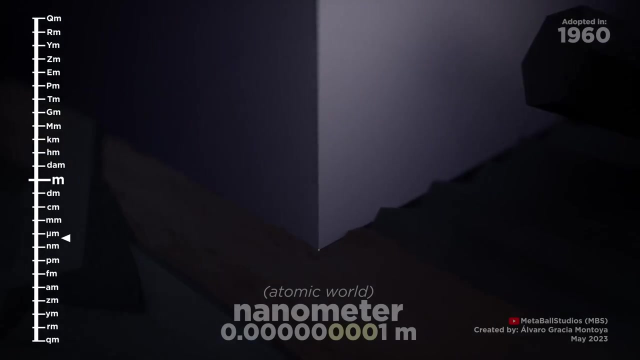 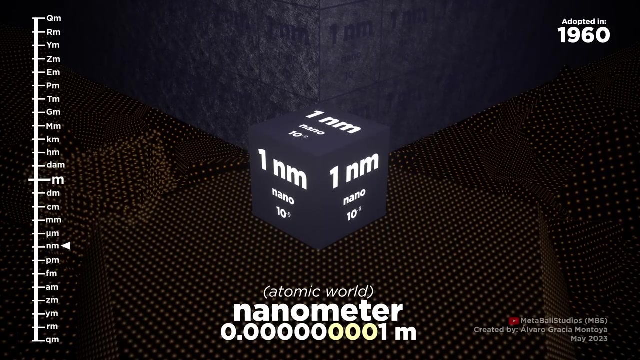 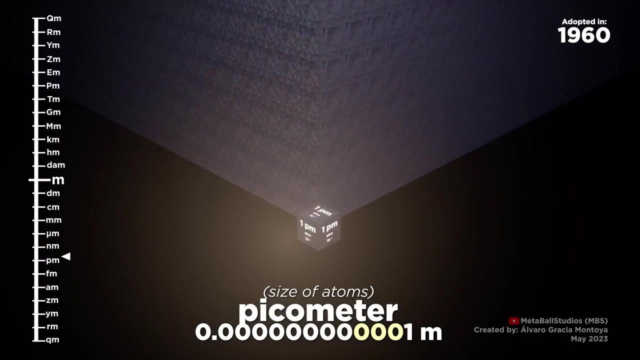 In the following we will represent all the existing prefixes representing it from a cube of one meter long, with one square meter each face and one cubic meter of volume. In the following we will represent all the existing prefixes representing it from a cube of one meter long, with one square meter each face and one cubic meter of volume. 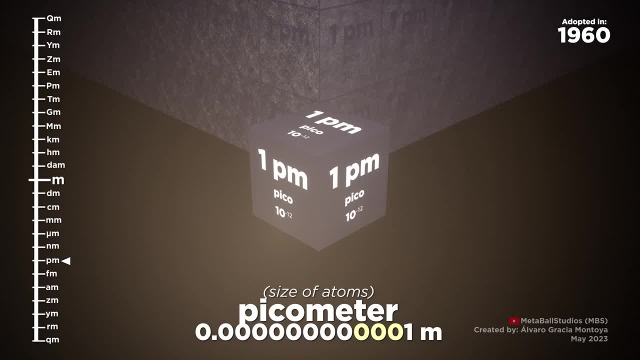 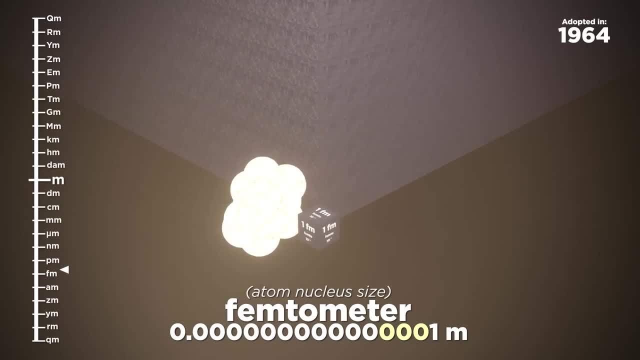 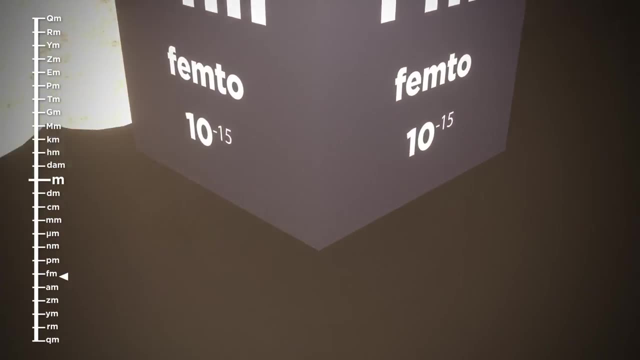 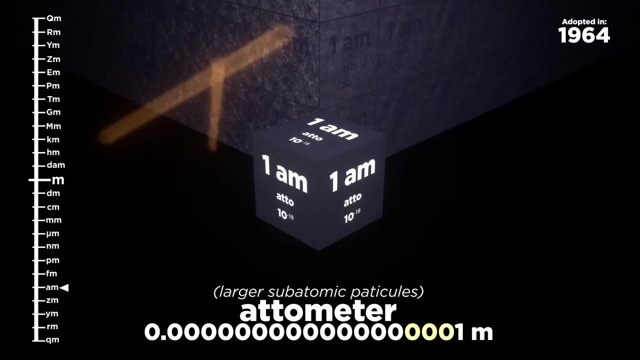 Here we have gradientsander parar. We will introduce stars, We willchiovers INCline on the optical axis athletes ції, ERT, Pericris, FRI, 첨 ade CP Cannons. 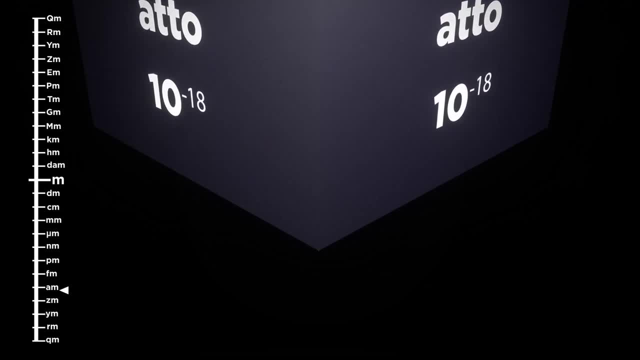 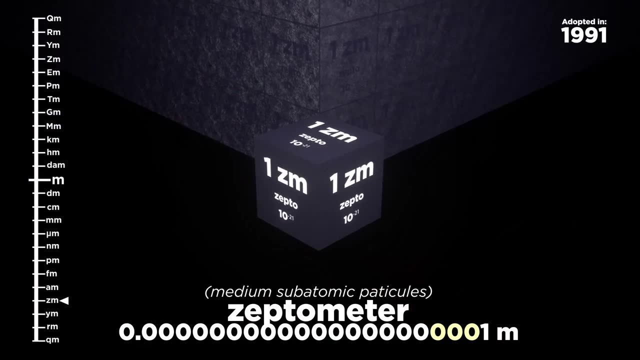 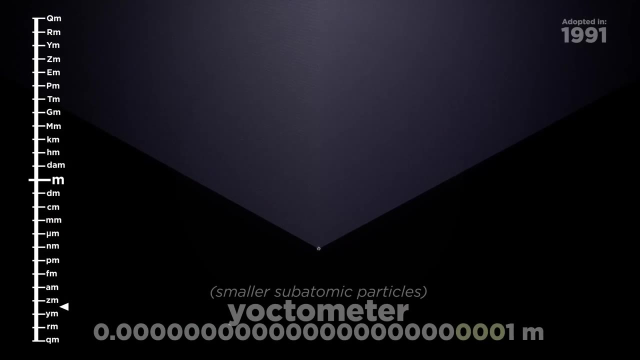 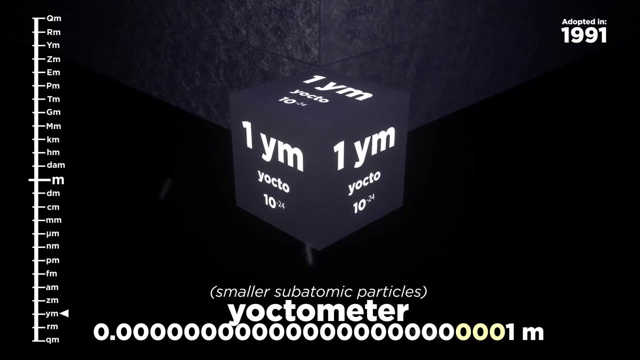 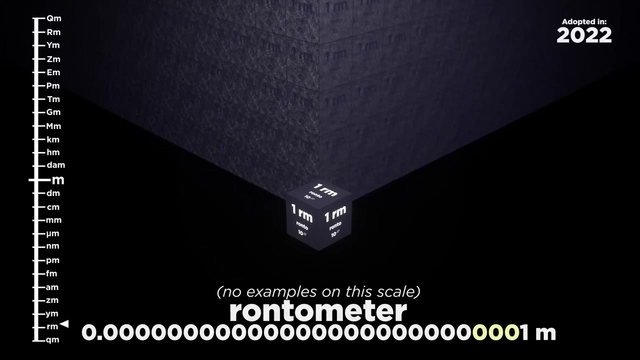 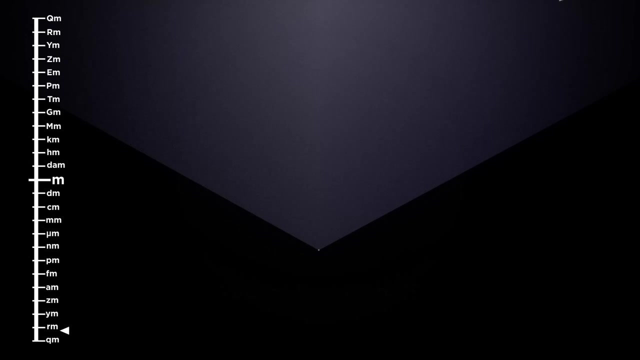 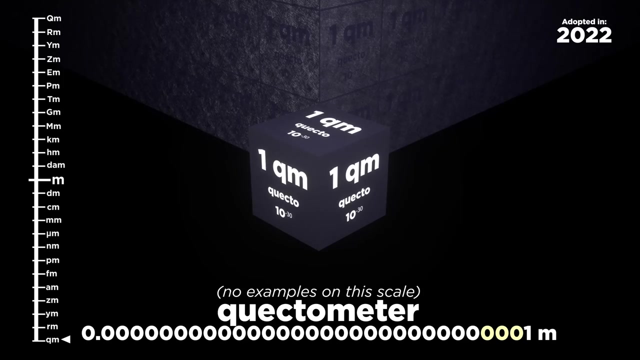 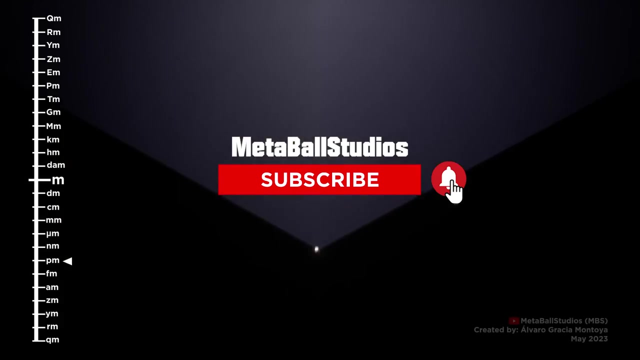 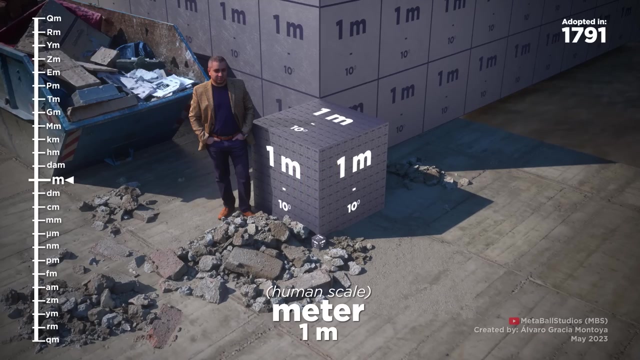 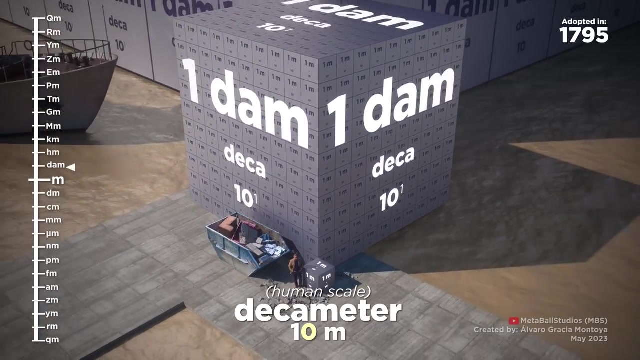 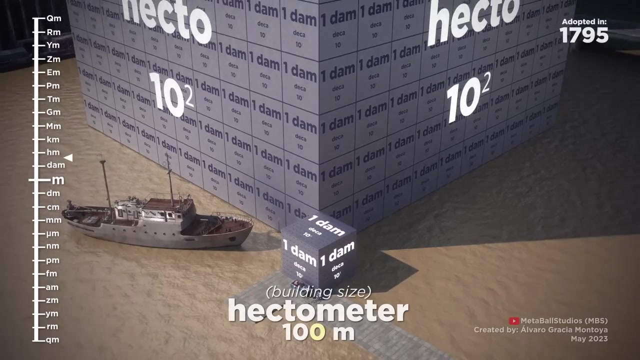 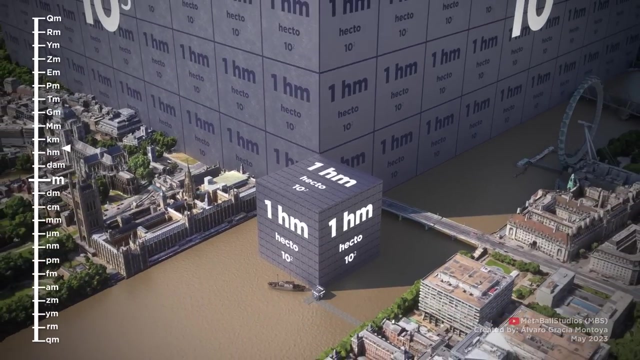 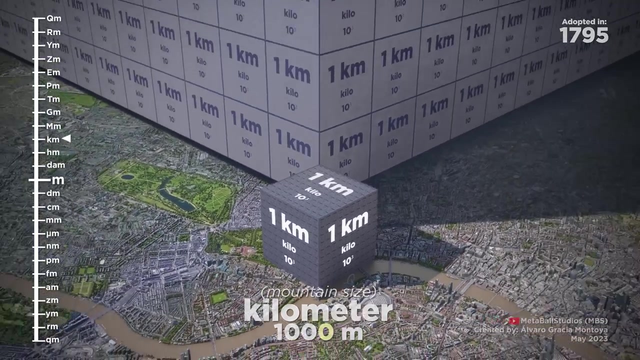 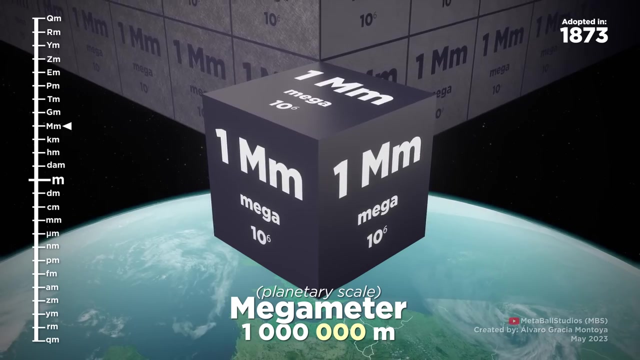 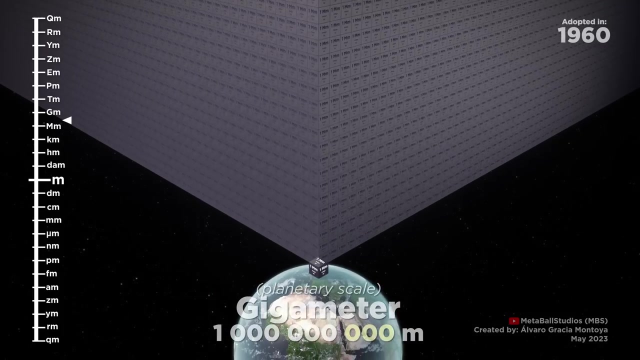 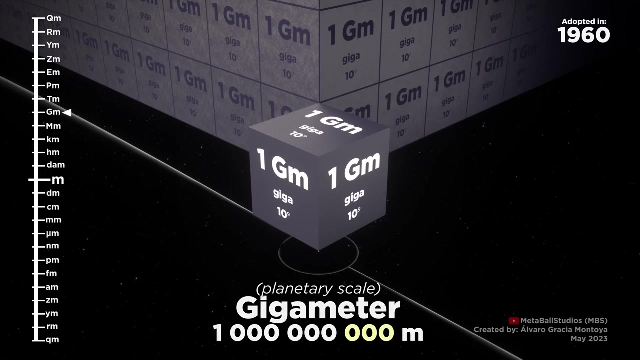 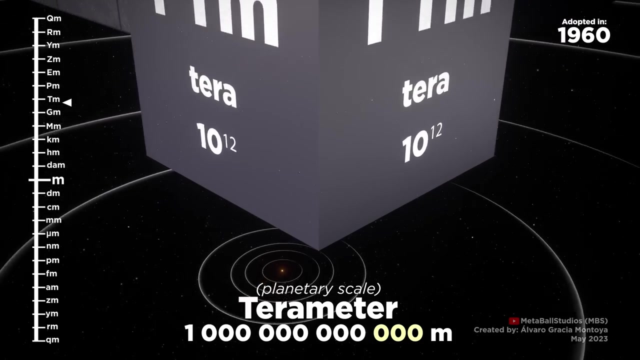 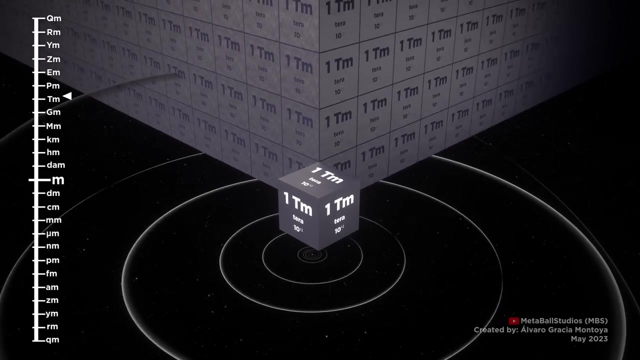 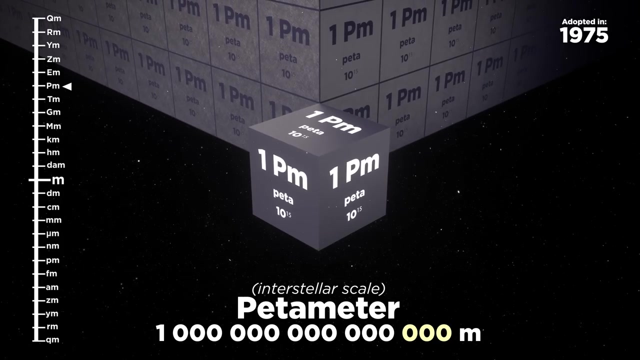 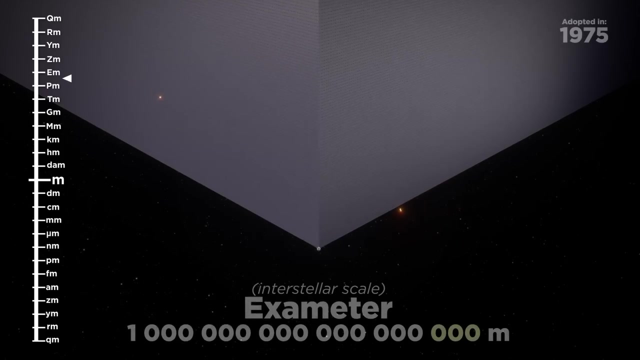 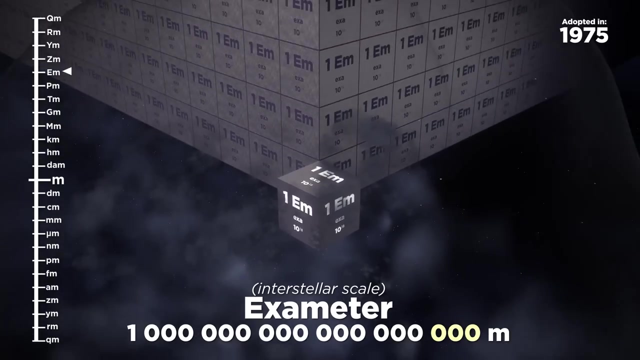 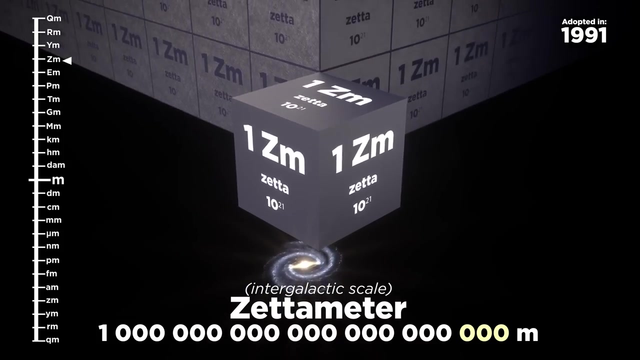 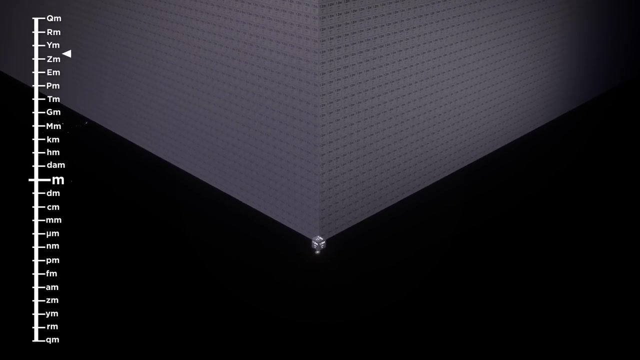 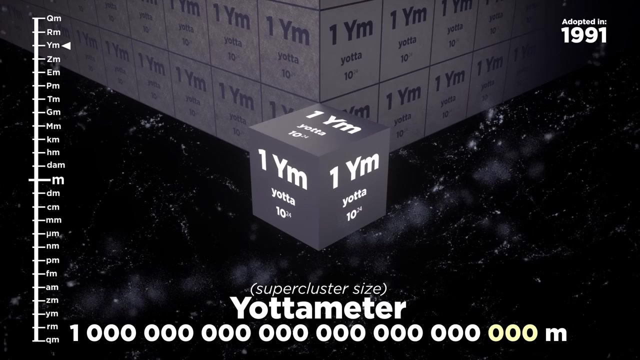 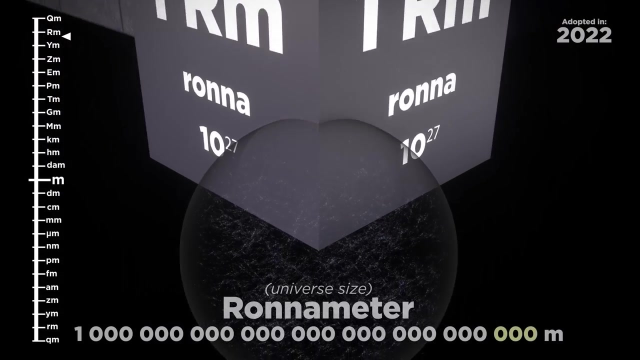 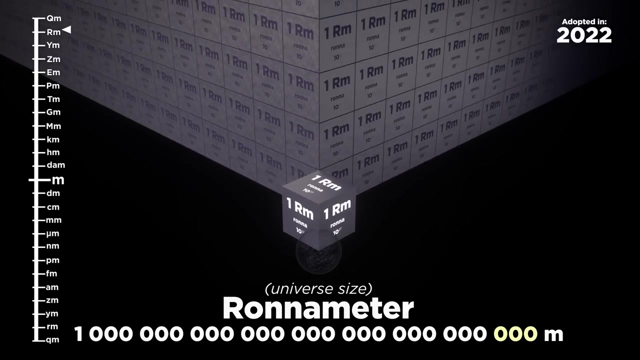 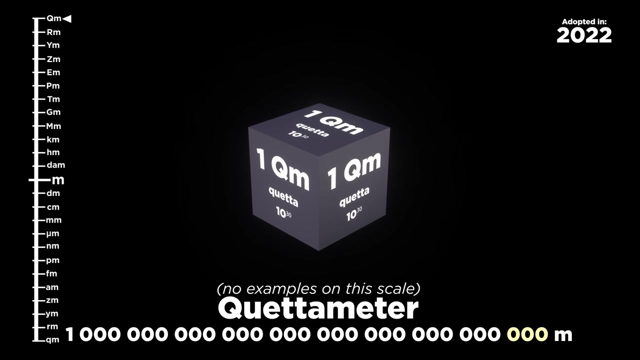 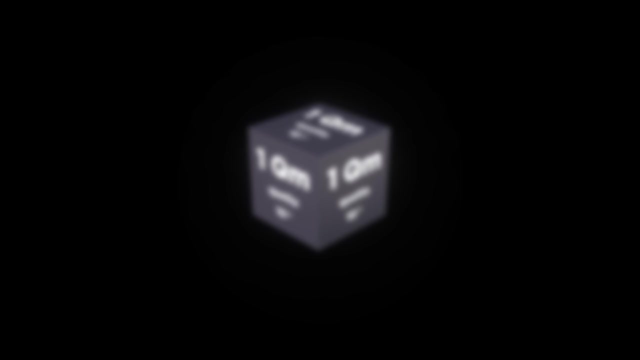